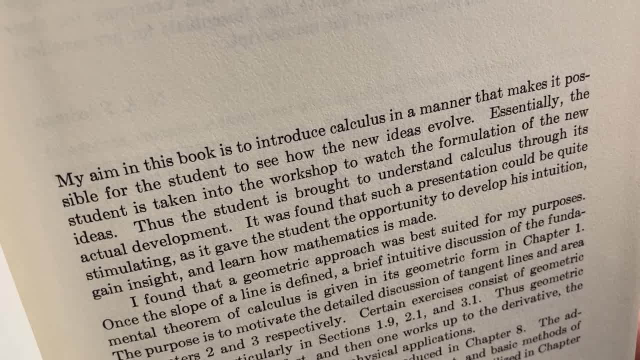 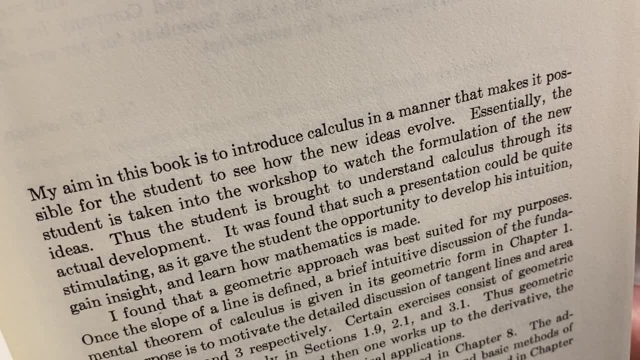 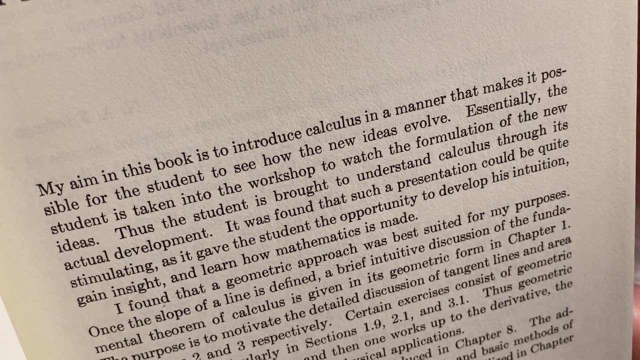 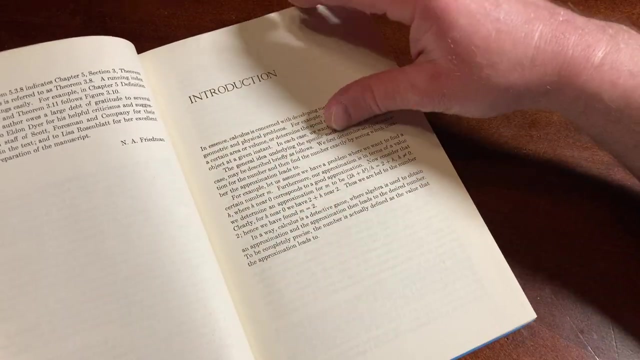 My aim in this book is to introduce calculus in a manner that makes it possible for the student to see how the new ideas evolve. Essentially, the student is taken into the workshop to watch the formulation of the new ideas. Thus the student is brought to understand calculus through its actual development. Hmm, Interesting. Here's an introduction Description of the text. 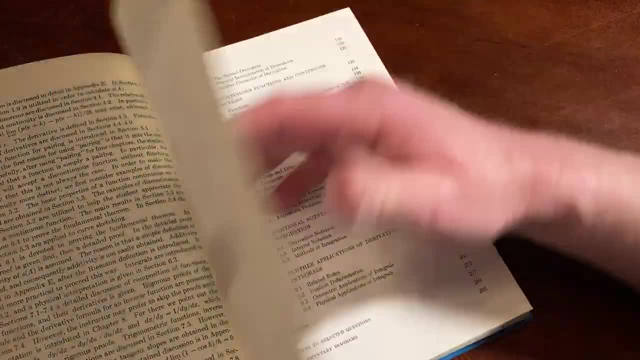 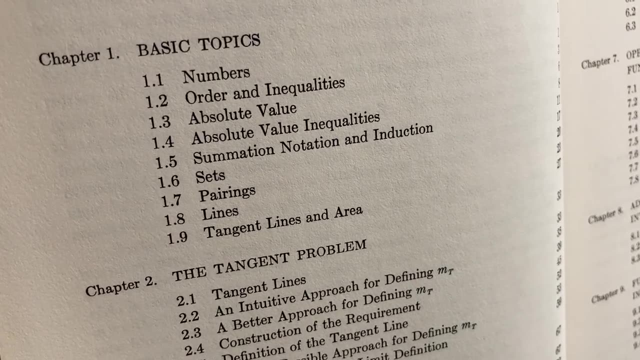 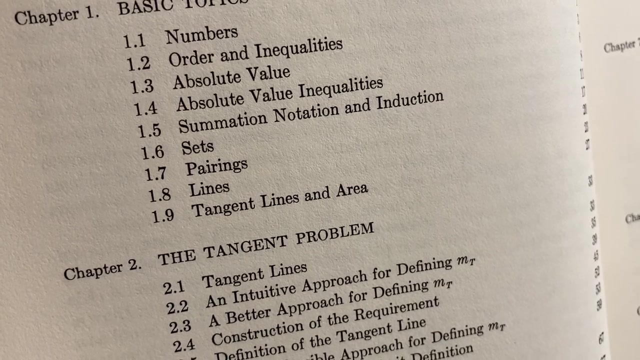 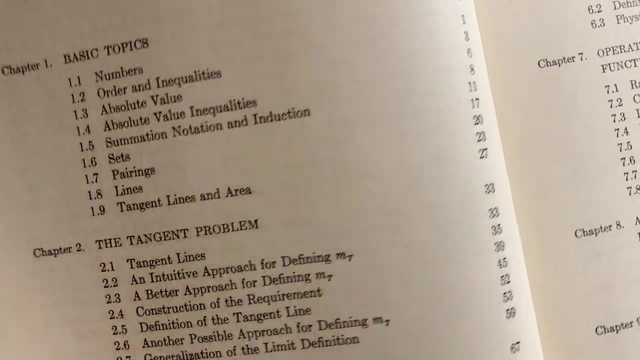 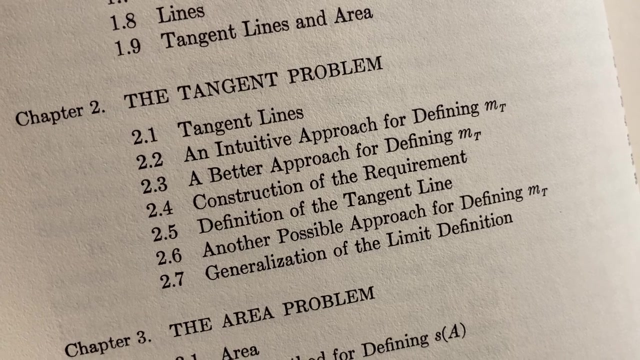 All right, Let's just Jump to the contents. See what we got. Contents: Here we go. Chapter 1. Basic topics. So numbers, Order and inequalities. Absolute value- Very important Absolute value, inequalities, Summation, notation and induction Sets, pairings, lines- That's a lot of stuff. Tangent lines and area- I mean, that's a lot of content. So quite a bit. 27 pages. Okay, The tangent problem, Tangent lines, All right. 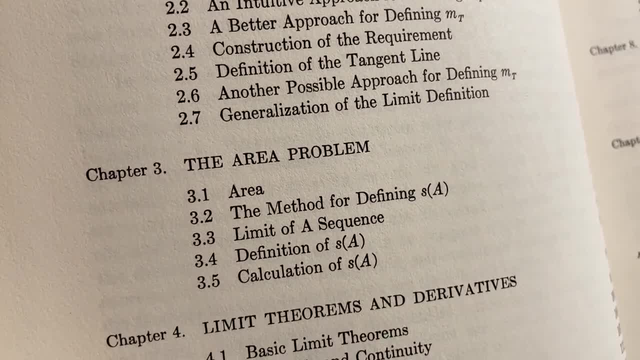 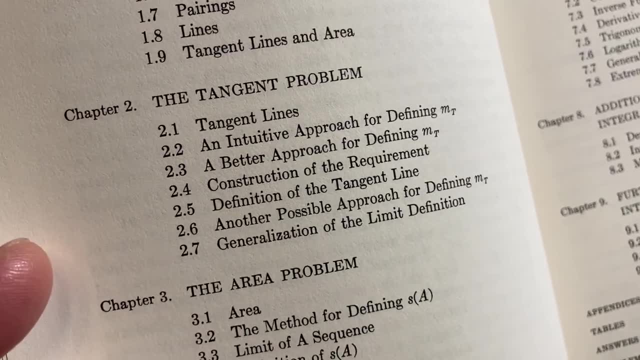 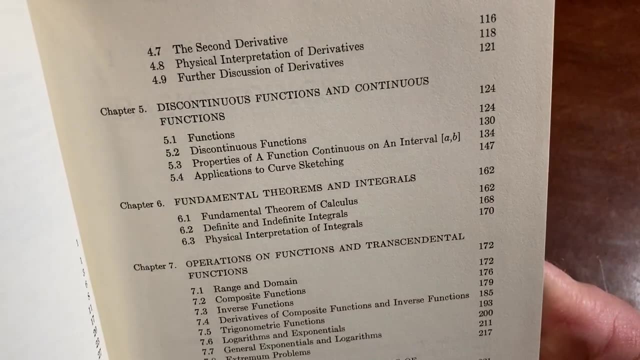 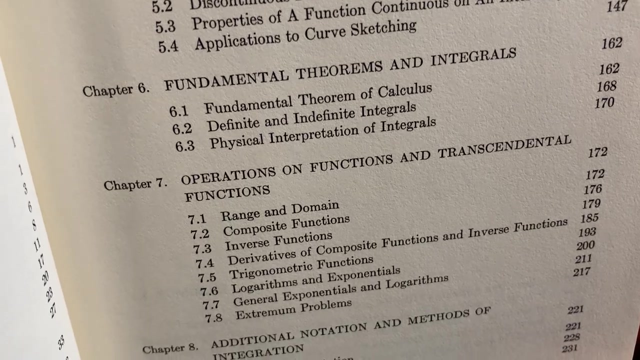 And then the area problem And then limit theorems and derivatives. So it's interesting. So they introduce these two big problems first and they spend a lot of time there and they develop that. That's cool. Just continuous functions and continuous functions, Fundamental theorems and integrals, Operations on functions and transcendental functions. 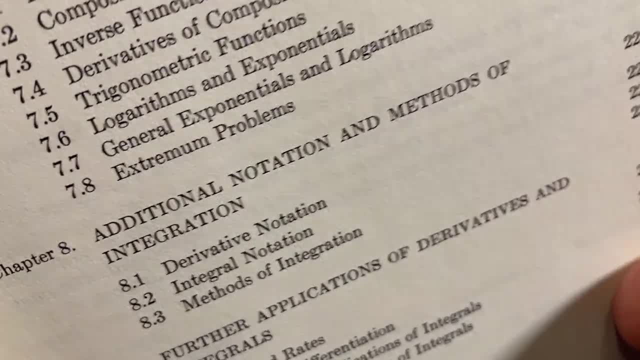 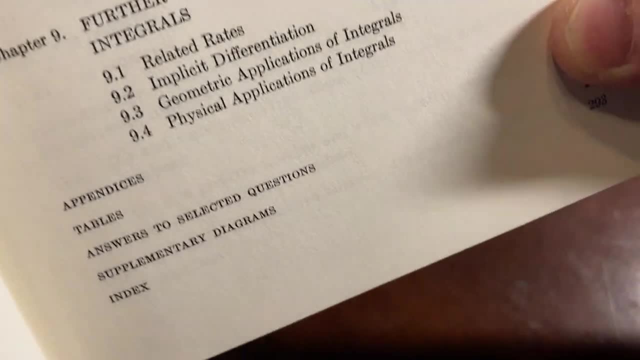 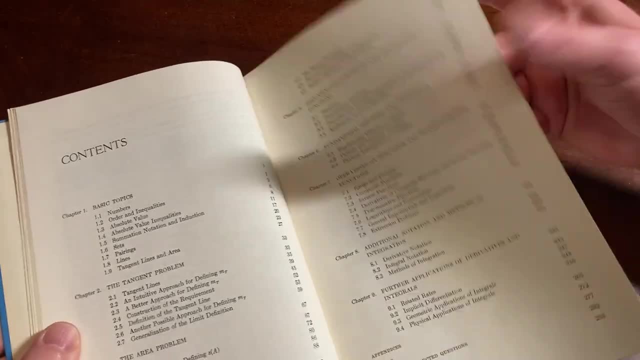 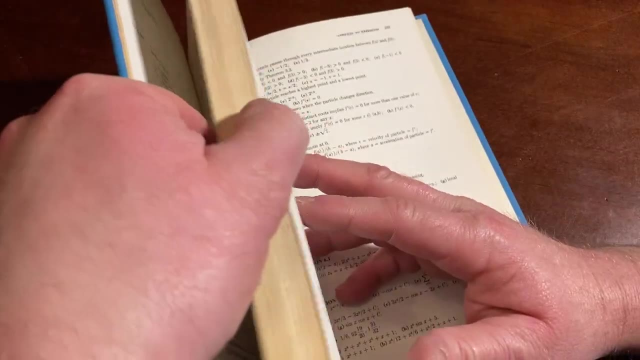 Okay, Okay, Okay, Okay, Okay, Let's go straight. Let's go straight to the answers, because I'm really curious to see what's there. So 277.. I'm just really curious to see what we have here for answers. 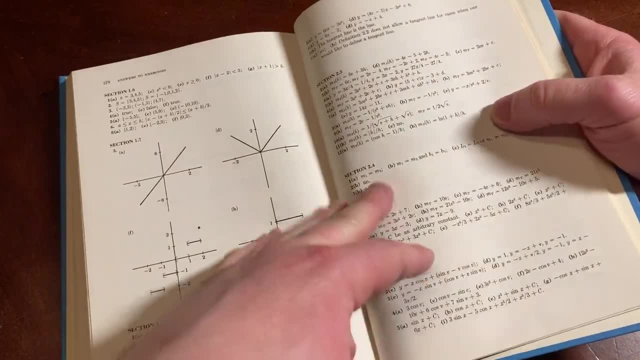 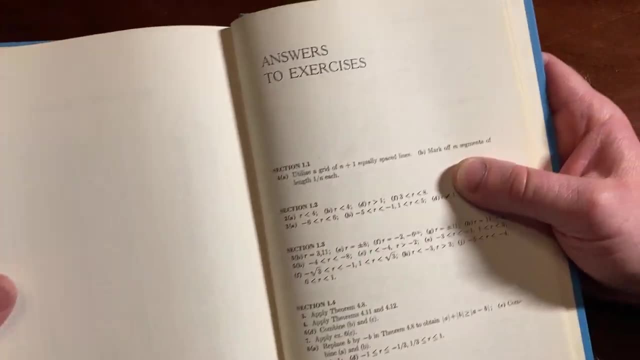 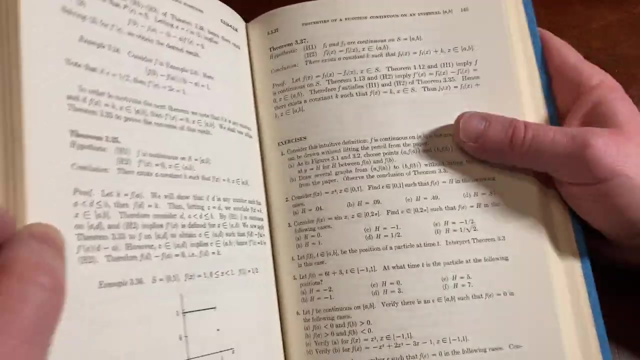 So look at all this. This is great, there's tons of answers. That's pretty cool. you know, not everything is here. It just says answers to exercises, but they're not all there. so yeah, Yep, it should say selected exercises. 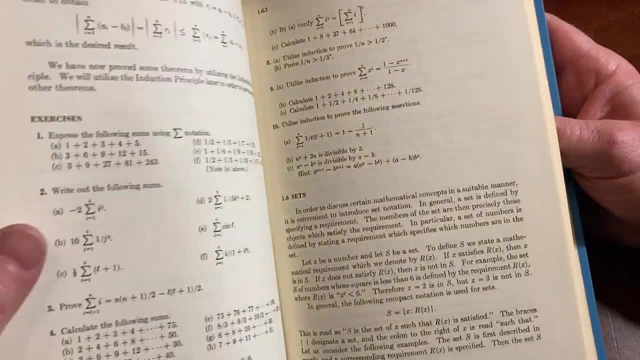 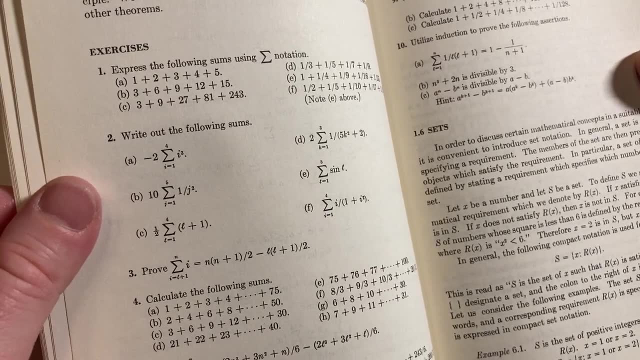 or something to indicate that they're not all there, or some exercises, so I don't know. Oh, interesting, so you've got some exercises here and we don't have answers to all of them, though, but you still have answers, so that's good. 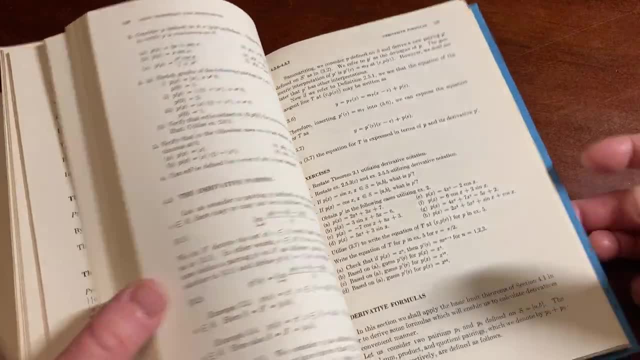 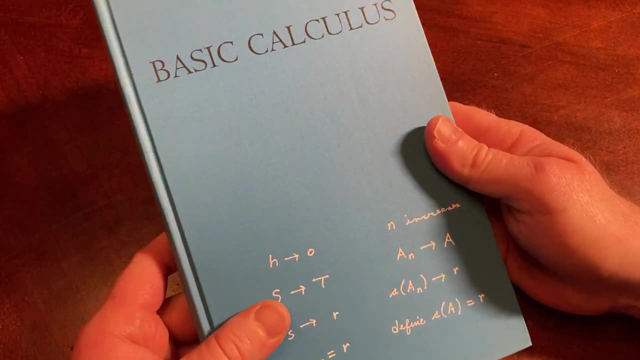 I like a few things about this book. so first of all, the feel. I just gotta smell it. I just ah, it smells really good. It reminds me of a book I have on abstract algebra by Hiram Palais, and I forgot the other author. 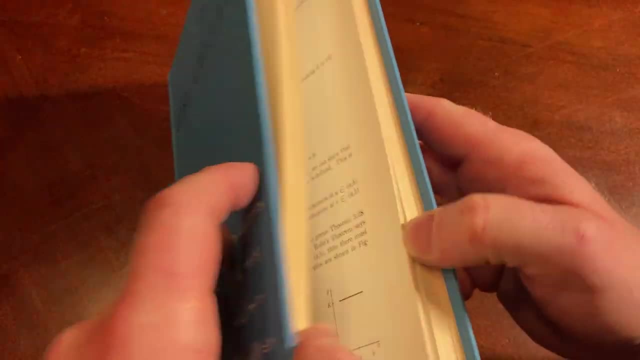 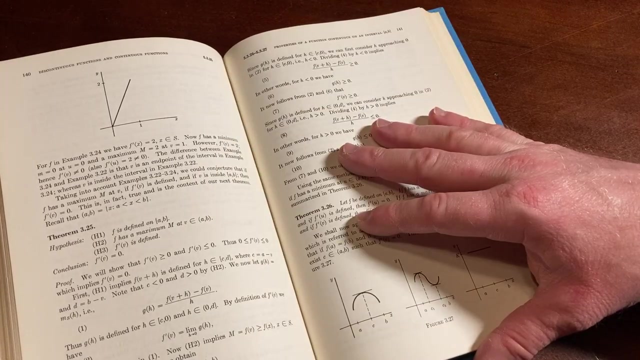 I just know the one author was Hiram Palais and it's an out-of-print book. You can't even find it on the internet, It's not. it's hard to find, I think. And it's the same size as that one. 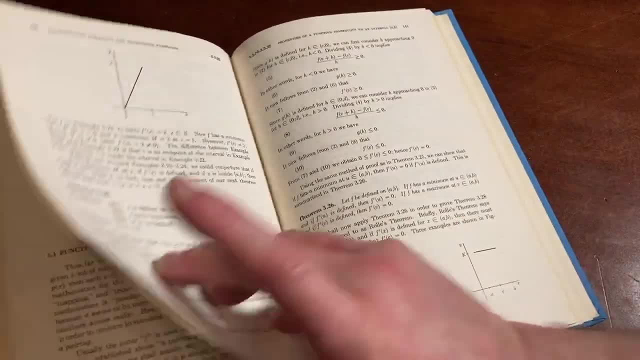 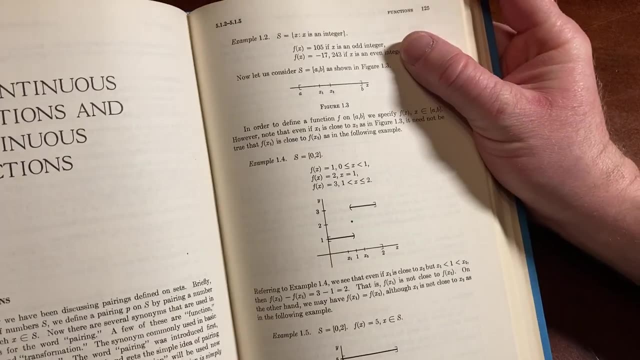 and it has the same smell, so different topic. but So this is interesting. Discontinuous functions and continuous functions- okay. So they have some examples here. Here's an example of a piecewise function. Okay, that's discontinuous, yep. 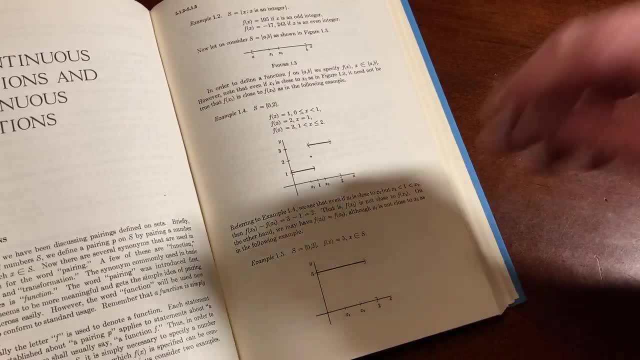 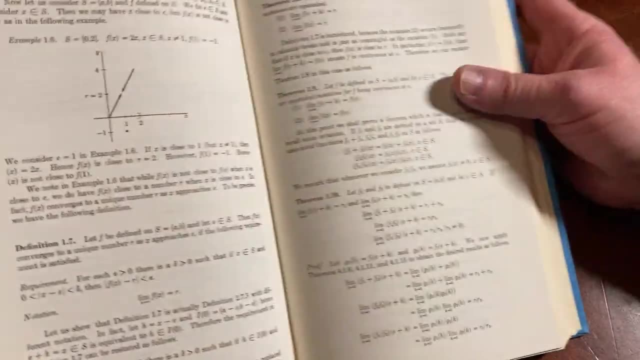 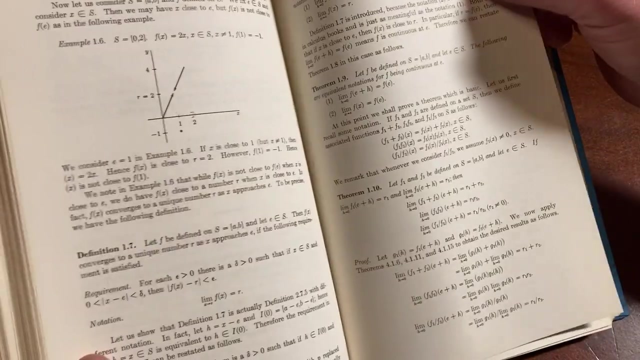 That's discontinuous at one. Basically, intuitively, it's continuous. if you could take a pencil or a pen and draw it without picking up your pencil, That's the basic idea of you know what a continuous function looks like. Huh, here's some more, some more mathematics. 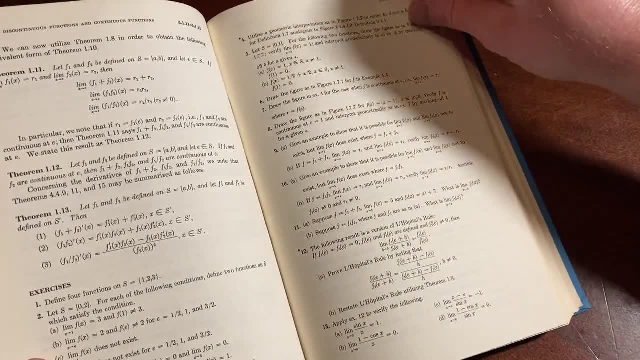 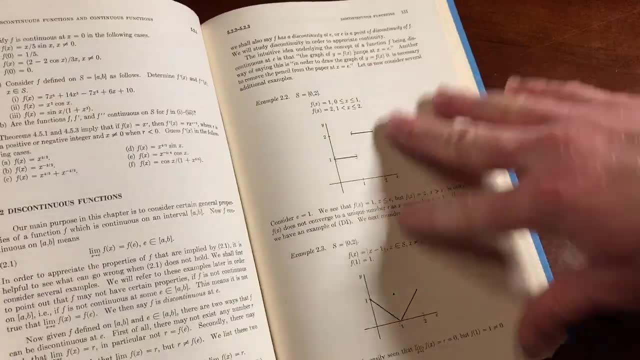 And then you have some exercises, Quite a few exercises. It does a really good job with the exercises, right? But again you only have some answers. That's but not a ton of examples in that section. Here's a couple here. 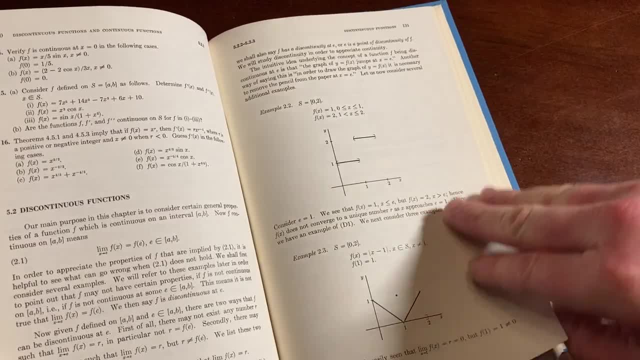 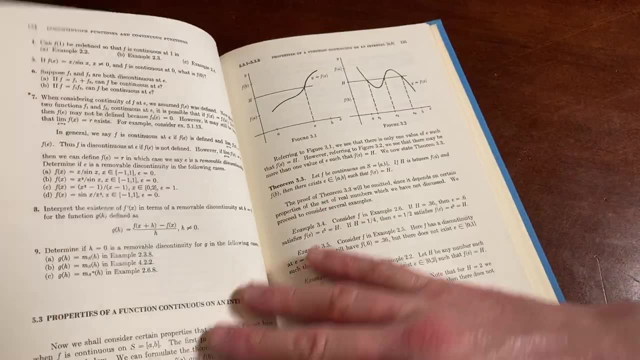 Here's two examples. it's pretty good: Piecewise functions. And then, oh, here's two more. Okay, so four. that's a lot of examples. That's four examples, That's pretty good. And then you have some exercises. 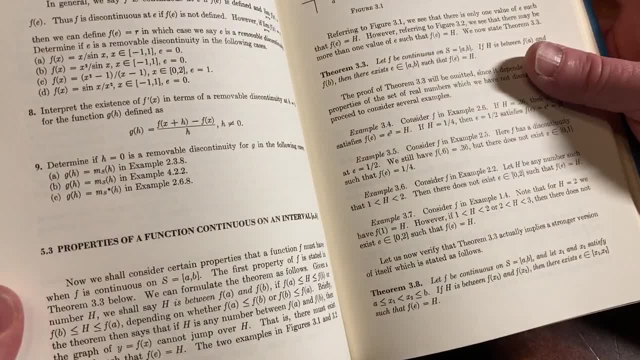 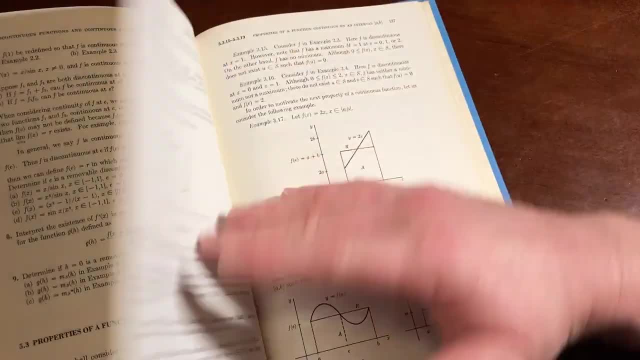 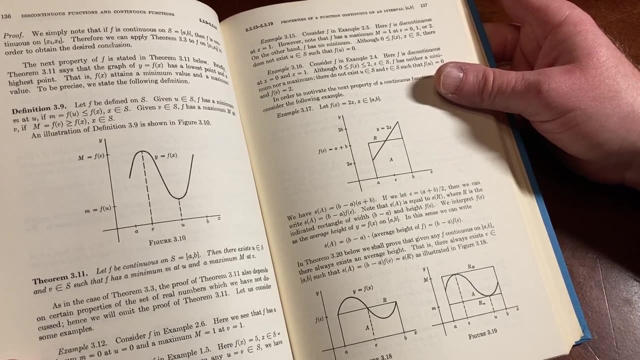 So here's a lot of examples, Properties of a continuous function on an interval a, b. Oh yeah, you can do a lot here. All kinds of fun, Lots of examples. Yeah, continuous functions are studied in calculus. So if you ever take calculus, you study those. 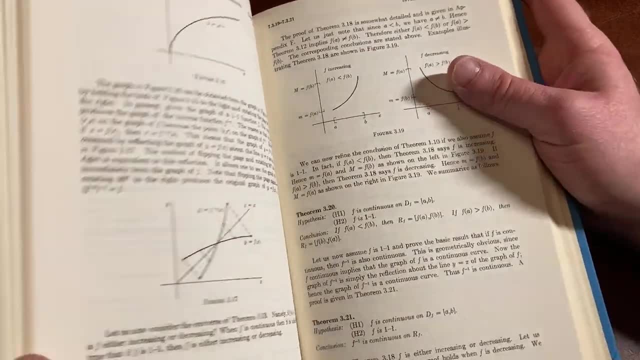 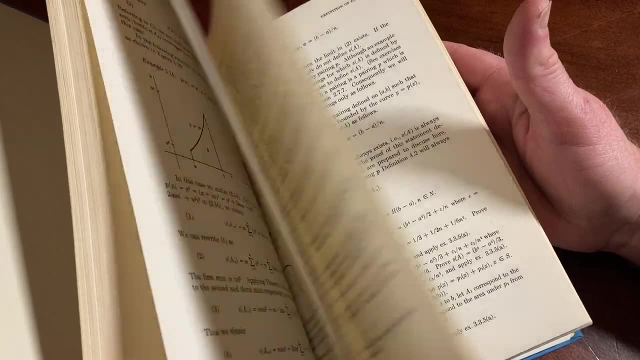 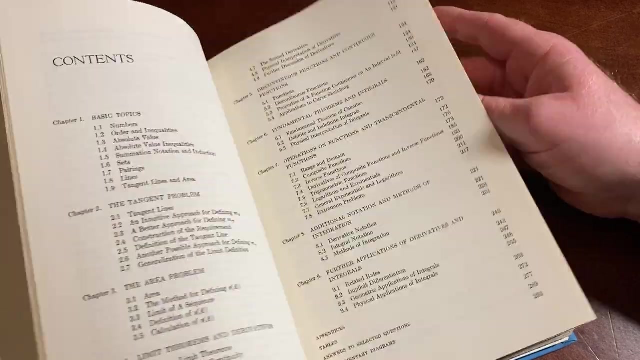 And yeah, they're just heavily studied. There's also things called uniformly continuous functions. There's also things called uniformly continuous functions- Cool. So this seems to be a pretty good book for self-study, but it would be better if it had 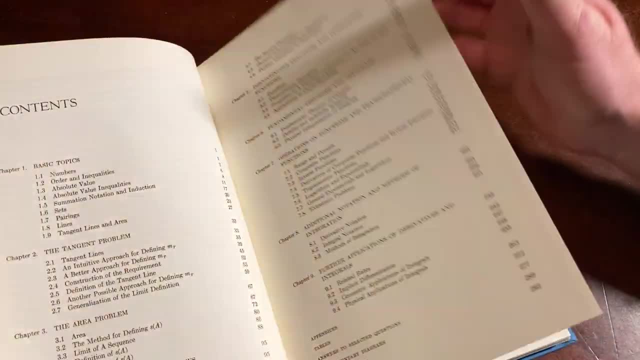 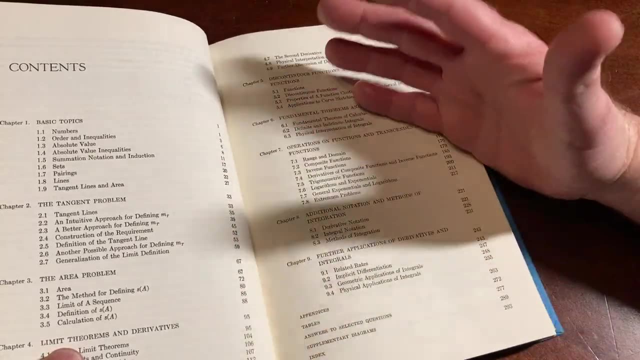 more answers. Also, I'm not trying to like knock the book and say it's bad or anything, but it doesn't have like. this is not. you know, you can't compare this to other books that have a lot more content. 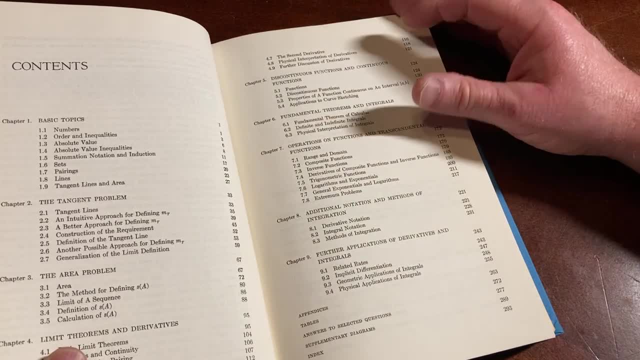 For example, there's no like there's no Stokes theorem in here. There's no. you know you can't compare this to other books that have a lot more content. For example, there's no like there's no Stokes theorem in here. 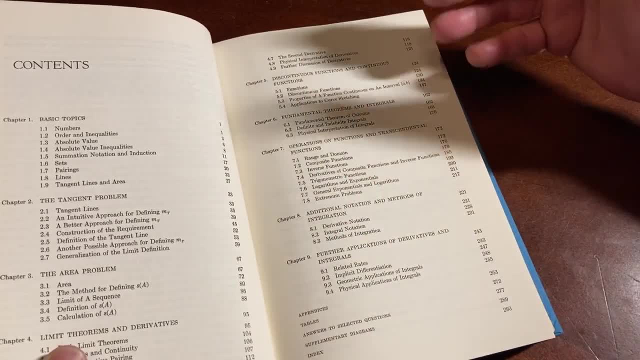 There's no Lagrange multipliers, There's no like multivariable, heavy, multivariable stuff in here. There's no like multivariable, heavy, multivariable stuff in here. It's all quite introductory, which is good. which is good. 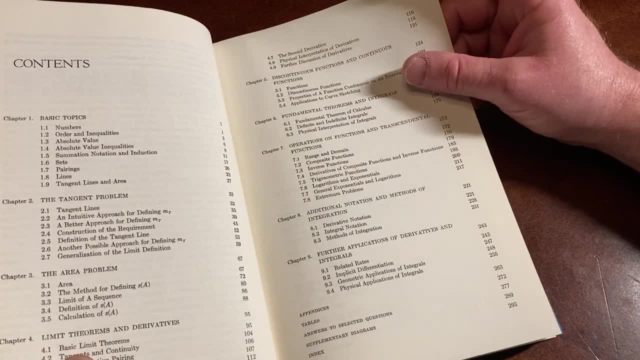 It does talk about other math a lot. I mean, it spends a lot of time. This whole chapter is on different types of math, which I think is kind of fun. I think it's a good thing to have in the book, especially: you know, you go out, you buy. 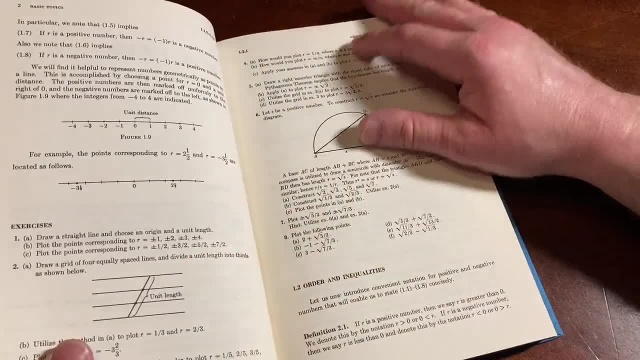 a basic calculus book. You think, okay, maybe it will help me get a little bit better at calculus, but then you have like this bonus chapter of like all this other math stuff and then you go to the next chapter and you're like, okay, this is more fun, this is more interesting. 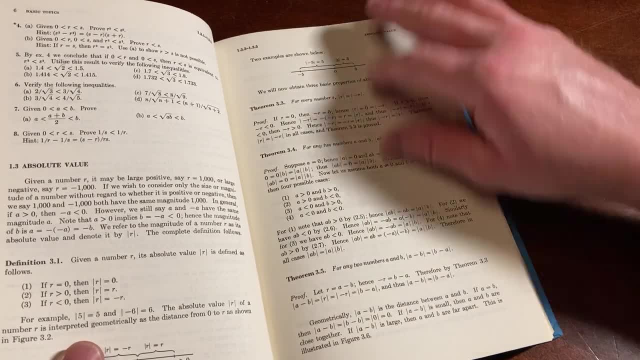 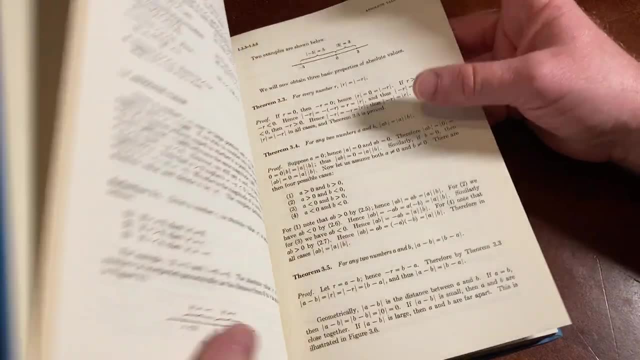 So that's why you look at this. I mean it spends a lot of time. This whole chapter is on different types of math, which I think is kind of fun. I think it's a good thing to have in a book, especially. you know you go out, you buy a basic calculus book. 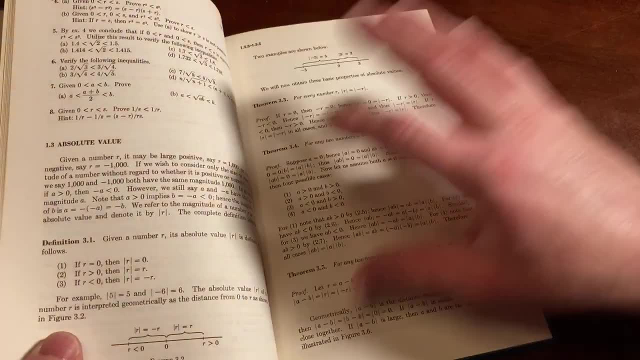 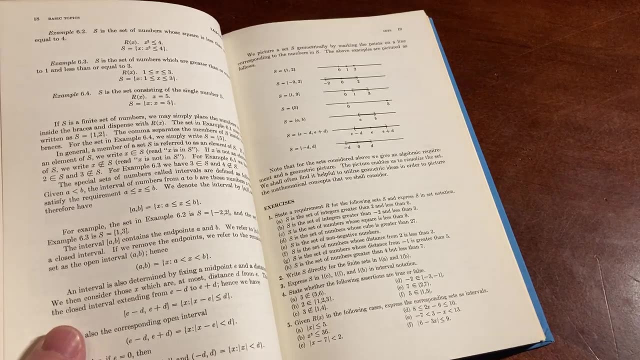 you think, okay, maybe it'll help me get a little bit better at calculus, But then you have like this bonus chapter of like all this other math. so I think it's great. That's one of the things I like about applied math books. 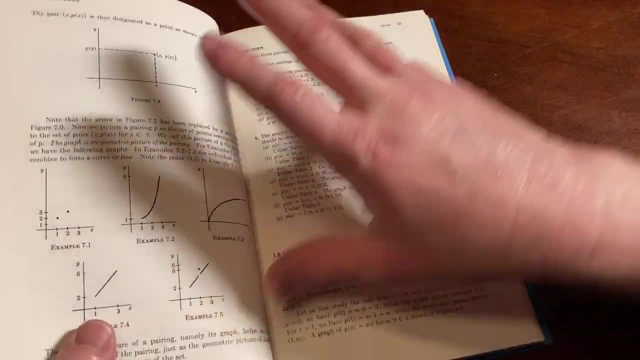 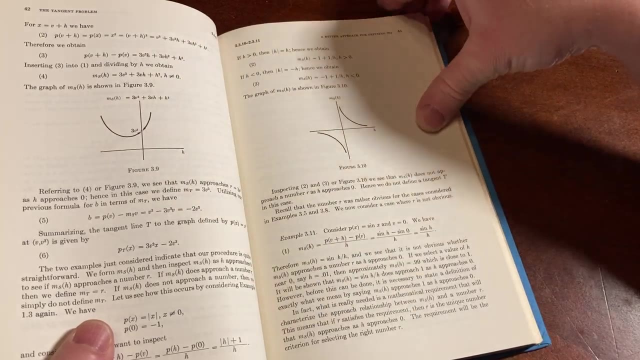 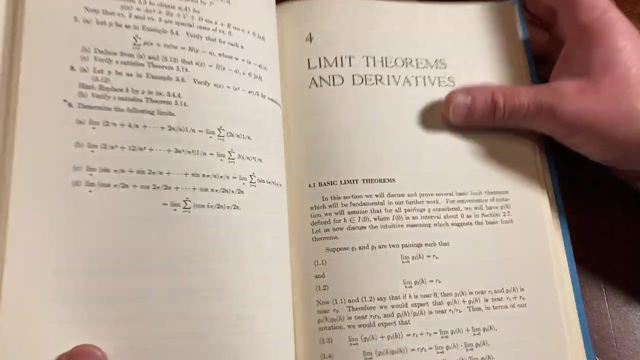 If you just get a book on applied math, a lot of times they have a lot of different topics and they're just kind of fun to look at because you'll have different fields of math in one book. So it's like lots of little introductory sections so you can get a taste for the different types of mathematics that is out there. 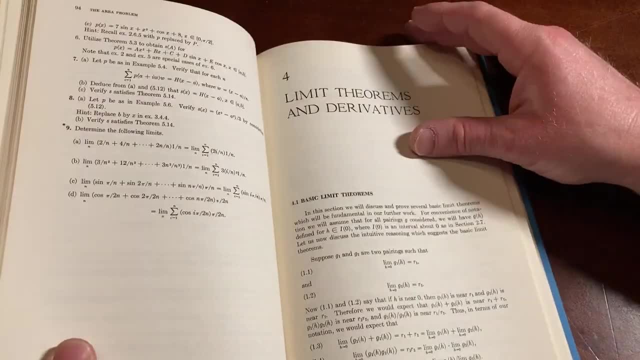 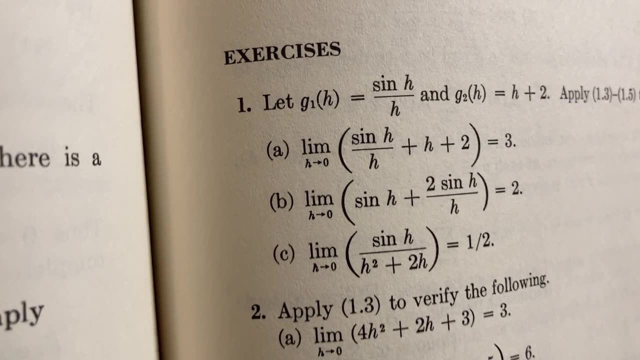 Limit theorems and derivatives. basic limit theorems. Let's look at some of the exercises here. Let's jump to the exercises. Let's see how hard they are. So here we go. exercises: Let: g of h equals sine h over h and g of h equals h plus 2.. 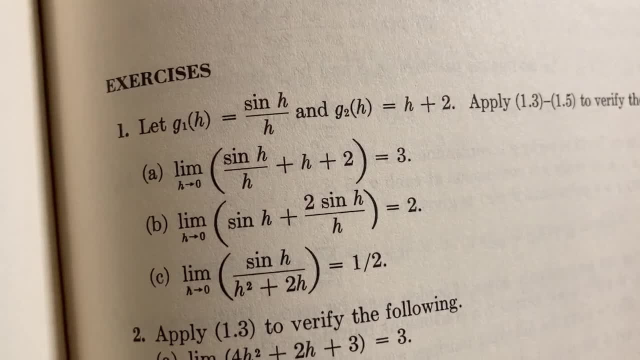 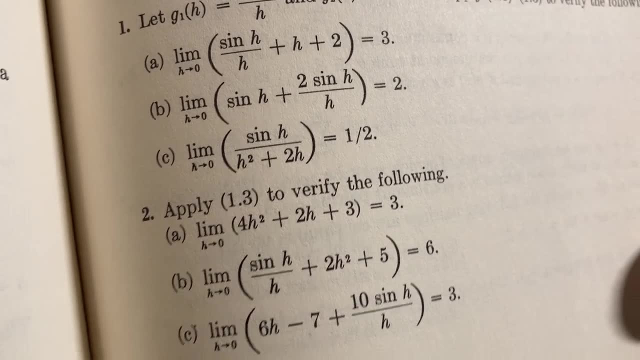 Okay, apply Those things to verify the following: Okay, so they're just having to apply the limit rule. That's really easy. I guess they want you to formally write it out and stuff. so there is like work to show, but it's really not hard. 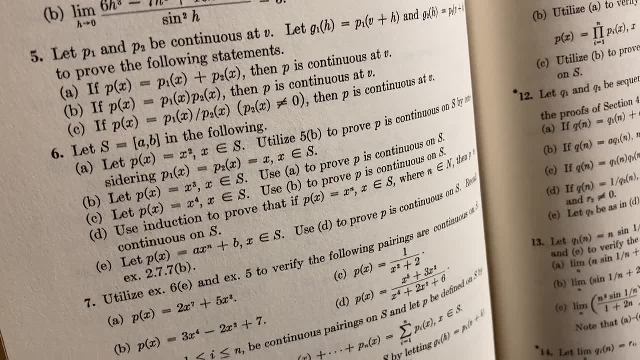 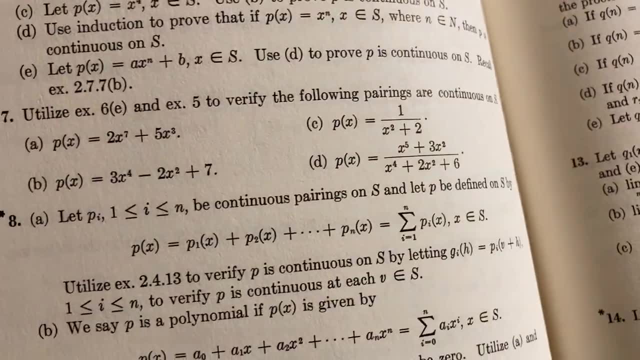 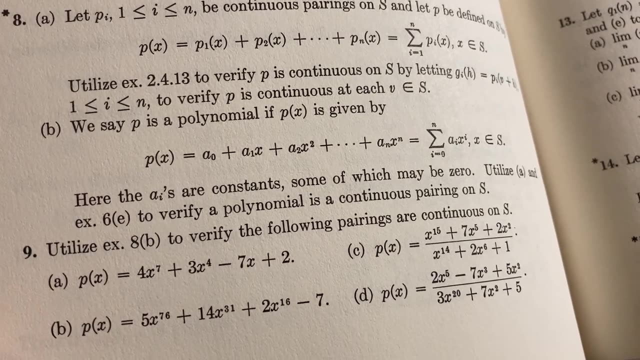 Let's go to the harder ones. Let's see: Utilize something and something. Verify the following pairs are continuous on: S, Let, p, Oh. If he's a polynomial, OK. Utilize example 8b to verify the following pairings: 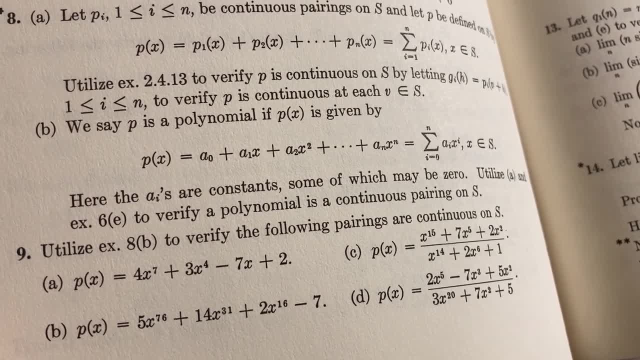 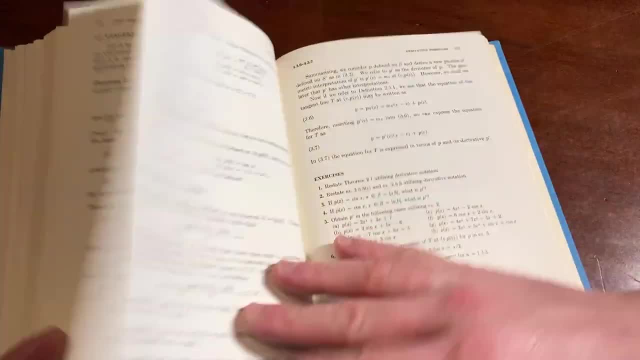 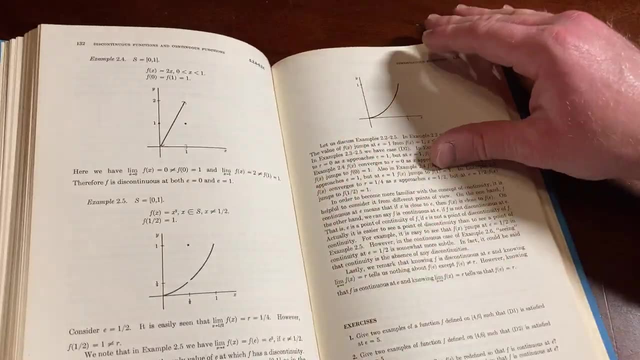 are continuous on S, So they want you to use some other examples to verify these things are continuous. So just a lot of conceptual stuff there, Nothing really. it's a little bit delicate. You have to think, right, You have to think, but it's not like. 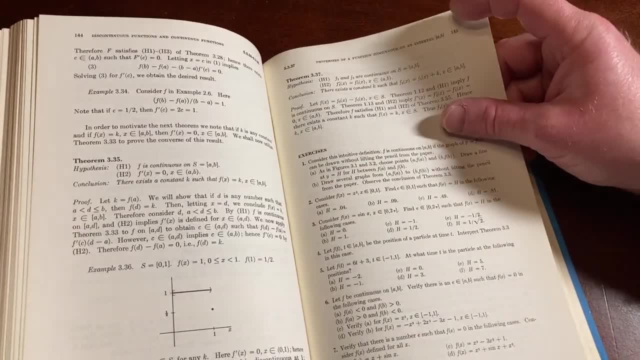 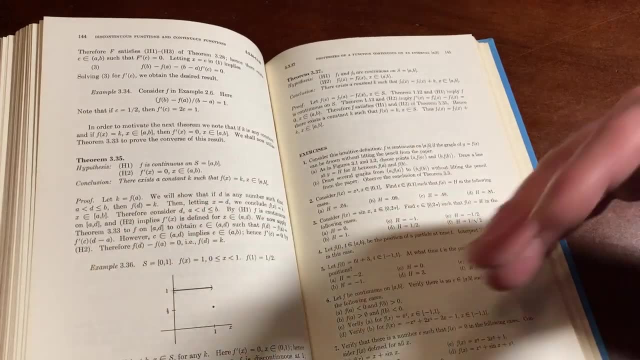 this reminds me of a book I have on. it's like a business calculus book And in the continuity section they have a lot of stuff. It reminds me of this book. There's a lot of focus on the conceptual which there are in other books. 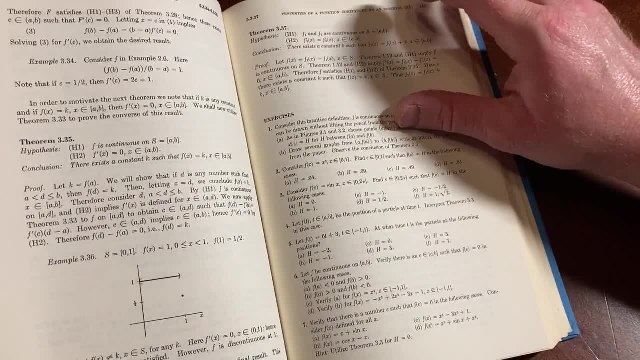 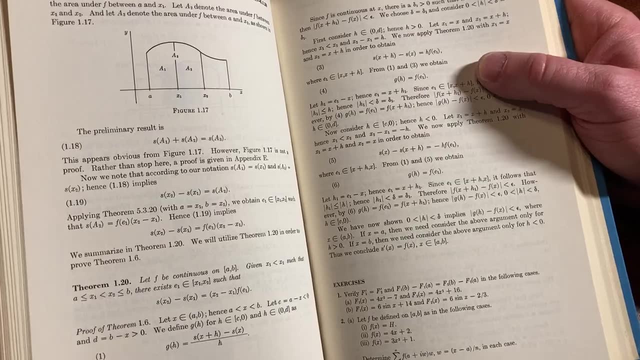 It's just. I feel like this one's spending a lot of time on that, which is good, Cool, Just different types of exercises. That's one of the things about getting different books right. You have different calculus books. This is very, very different from other calculus books.